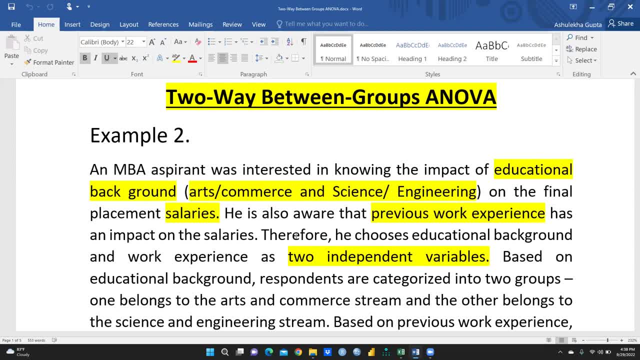 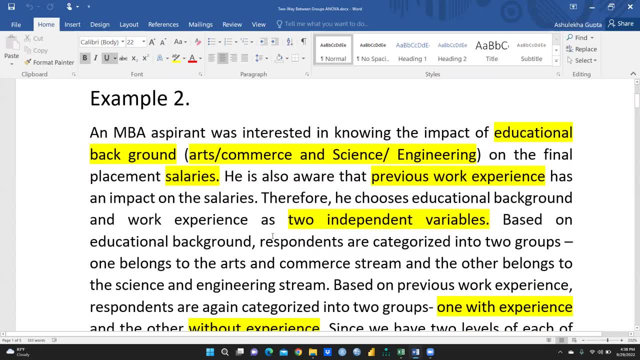 on the salary. salary depends upon all these kinds of qualification, So he is also aware that previous work experience has an impact on the salaries. Therefore he chooses educational background and work experience as two independent variables. Based on educational background, respondents are categorized into two groups. One belongs to: 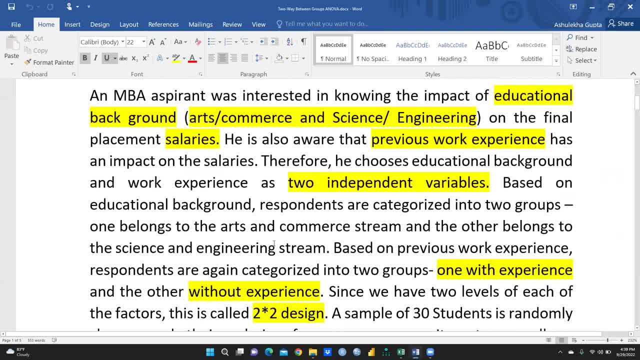 arts and commerce stream and the other belongs to the science and engineering stream. Based on the two-way ANOVA, one group takes the education background and the other belongs to the science and engineering stream. Based on the two-way ANOVA, one group takes the 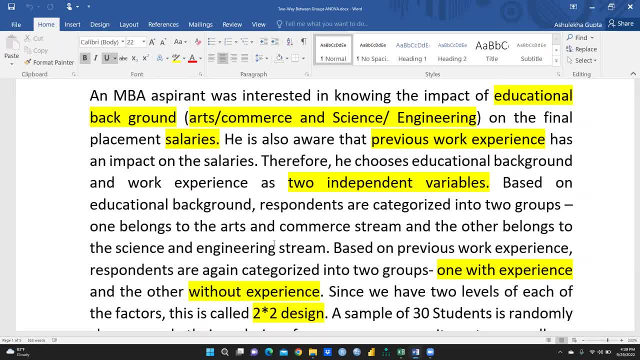 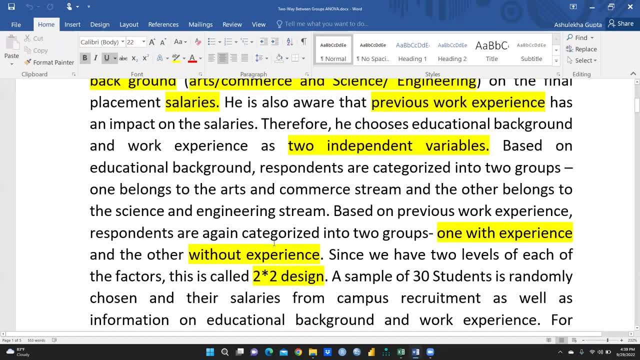 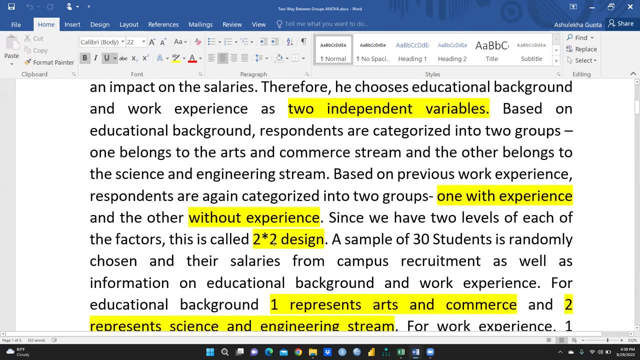 on previous work experience. respondents are again categorized into two groups: one with experience and the other without experience. Since we have two levels of each of the factors, this is called two by two design. a sample of 30 students is randomly chosen and their salaries from campus. 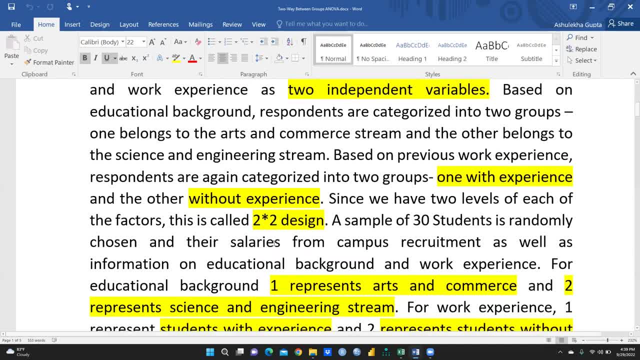 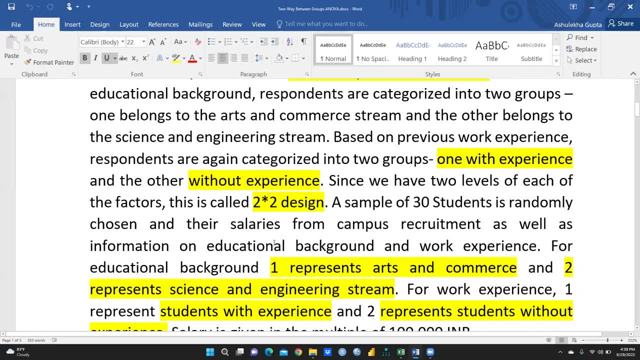 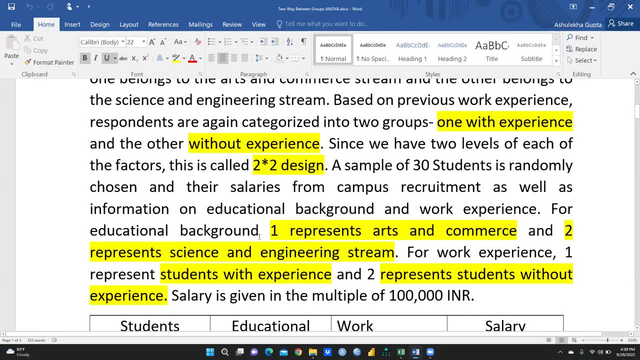 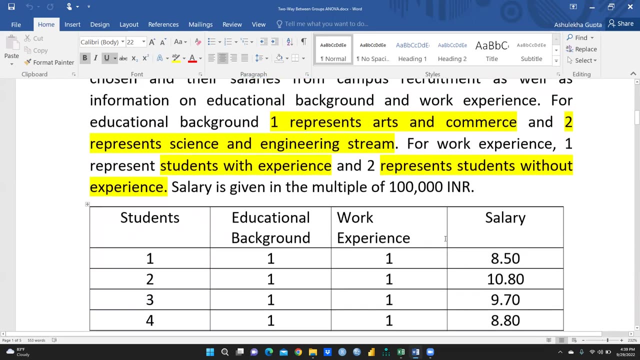 recruitment, as well as information on educational background and work experience. For educational background, one represents arts and commerce and two represent science and engineering stream. For work experience, one represents students with experience and two represent students without experience, and salary is given in the multiple of Lex. So here is- you can see total. 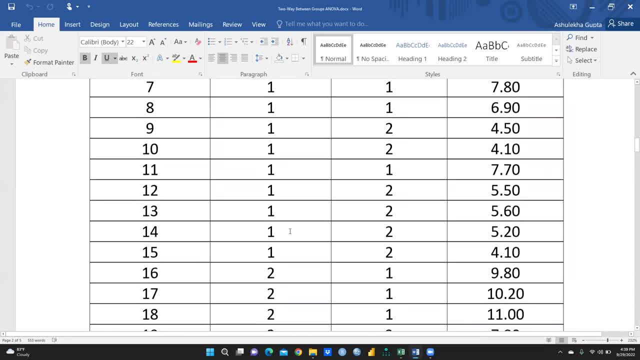 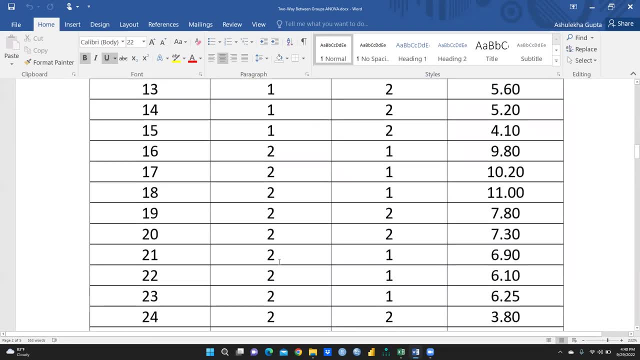 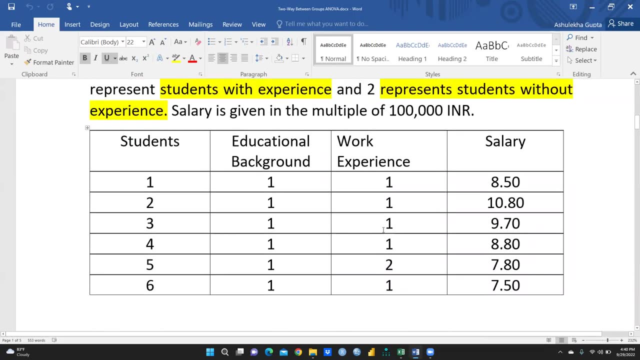 MBA aspirants data is 1. 30 students data. one means educational background they are. one means they are from arts and commerce background and two means they are they belong to science and engineering background. but when we talk about the work experience, one is transfer- they have work experience. two means they do not. 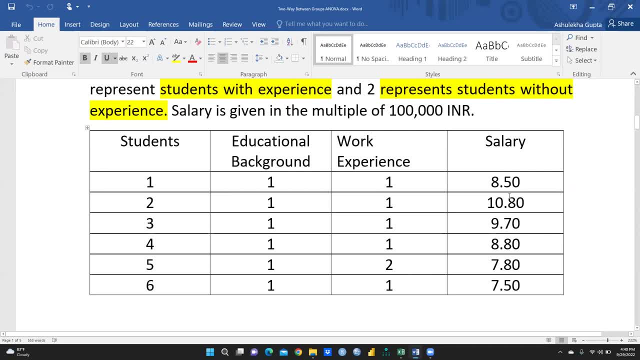 have work experience. so this is the salary what these students they are getting, with the combination of two independent, variable educational background and work experience, and that is multiple of lakhs. that means 8.50 lakh, 10 lakhs, 80 000, 9 lakh. this is the salary. so there is the hypothesis. 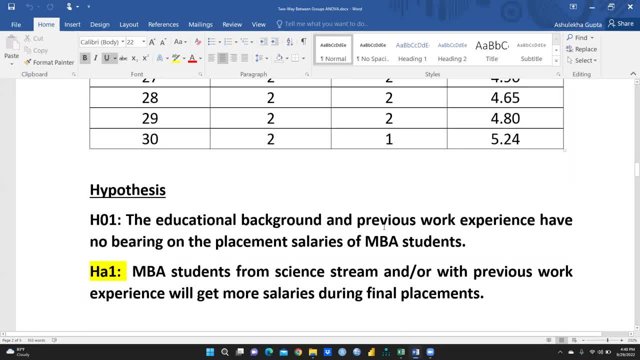 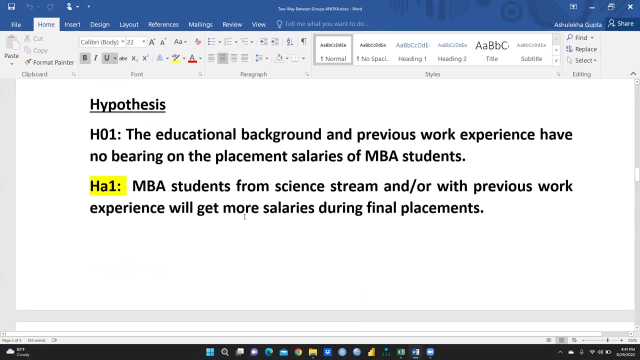 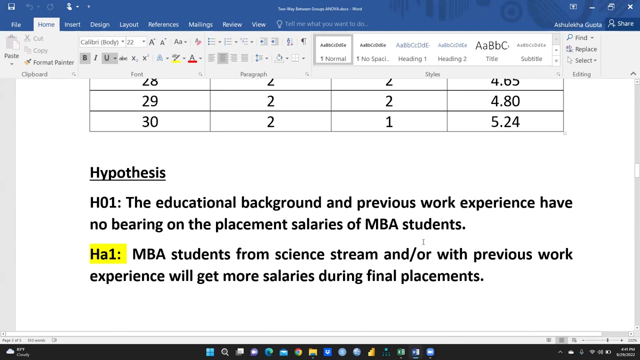 to hypothesis null means the educational background and previous work experience have no bearing on the placement salaries of mba students. but alternate hypothesis said mba students from science stream and or with previous work experience will get more salaries during their final placement. i have already explained you in my previous videos, through spss, this test, but today what 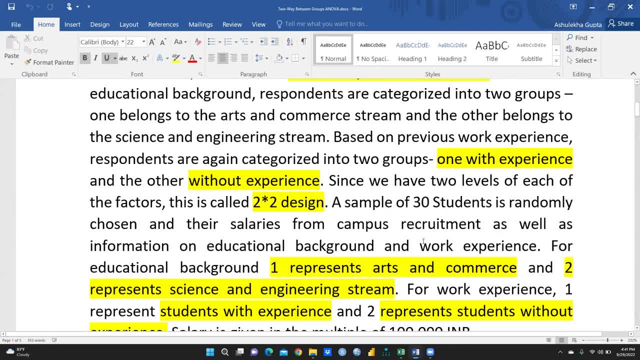 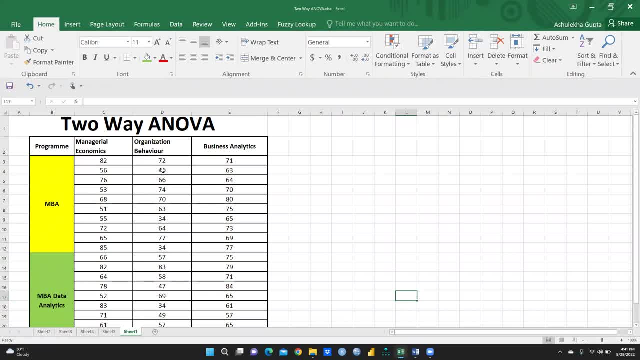 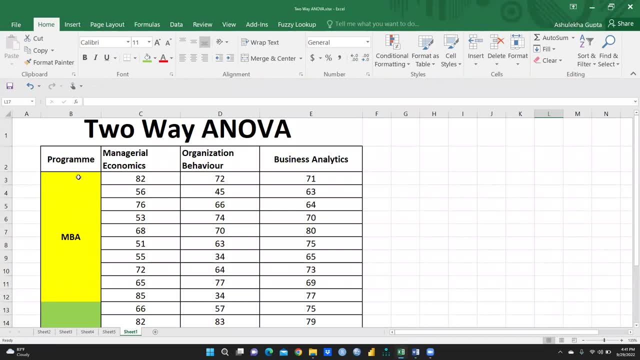 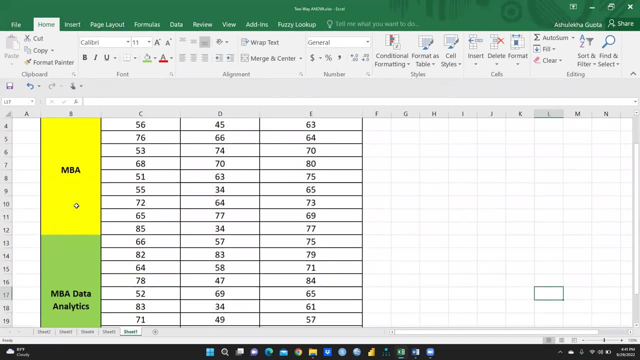 we have to do. i am just telling you two-way anova with the help of excel, but i have taken some different example. this is an example. let me explain you this example. first, two-way anova. there is two kinds of mba program or post graduation program we are running in our mba department. one is mba, another one is mba data. 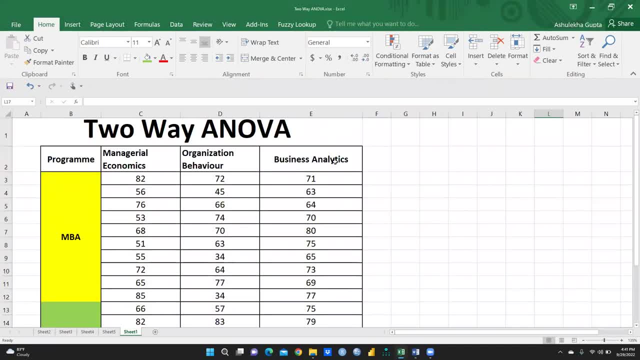 analytics. these are the three subjects. one is managerial economics, organizational behavior, organizational behavior and business analytics. these subjects, all both these programs, they are studying these three subjects and they are studying these three subjects. so these are the three subjects. it's hypothetical data, it's not real data and i just want to know there. 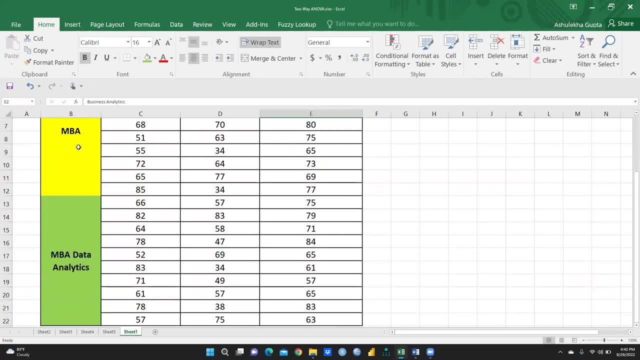 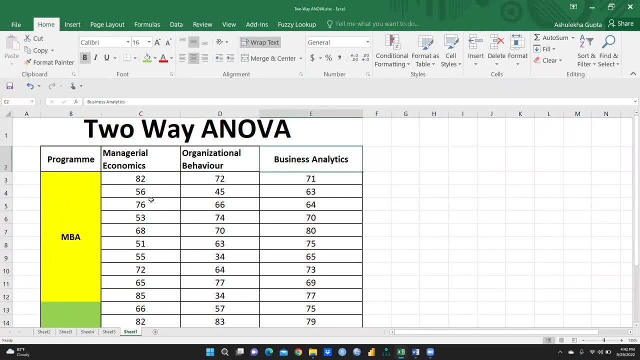 is any difference in between both these groups and as well as there is any difference in their marks. column wise also, and row wise also means there is the difference in between managerial economics marks and organizational behavior marks, organizational behavior marks, analytics marks or business analytics. managerial economics marks right and organizational behavior. 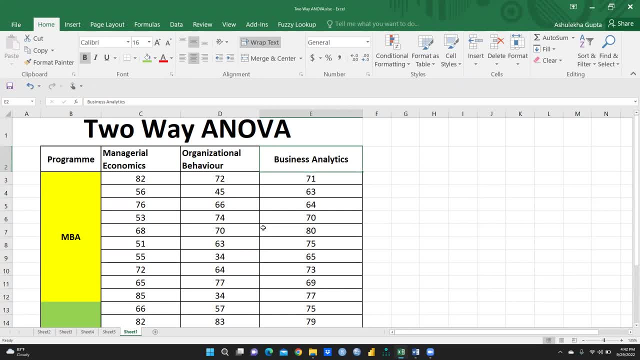 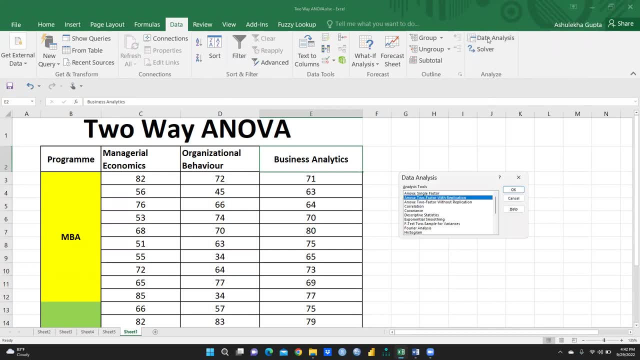 and business analytics marks. So I just want to compare all these things. So what I have to do? simply I will go to data and I will click here data analysis. and now you can see ANOVA single factor we have done. we had covered in my previous video ANOVA two factor with replication and 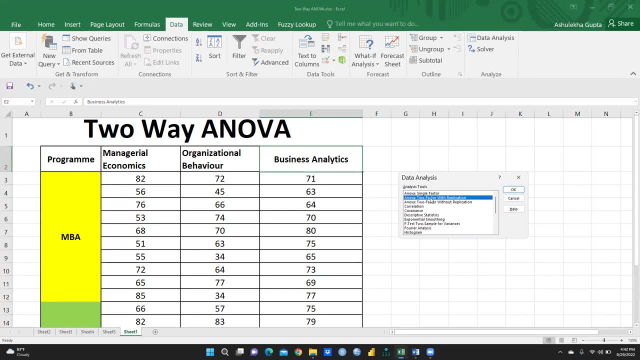 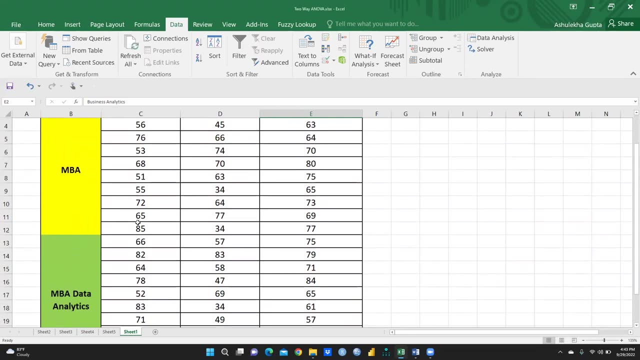 and third option is ANOVA two factor without replication. So here is when we talk about ANOVA two factor with replication means exactly equal data we have in MBA general program and in MBA data analytics. that means total number of. that is the replication of number of the rows Equal. 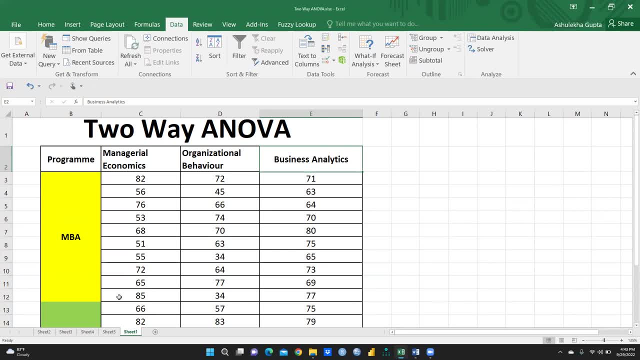 number of rows. I have 10 rows in MBA program, 10 students data and same is 10 students data in MBA data analytics. So what I will do? I just want to analyze simply, and I will use ANOVA, two factor with replication, because my data with replication, So I will not use ANOVA. 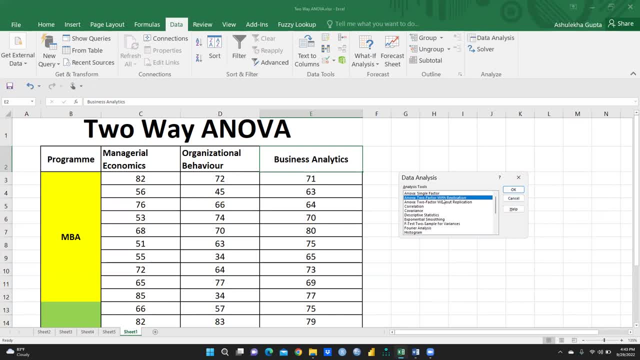 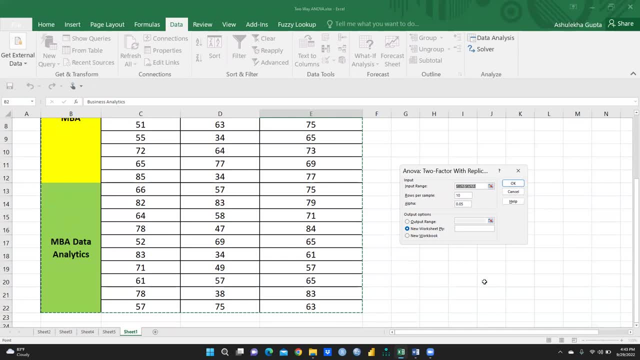 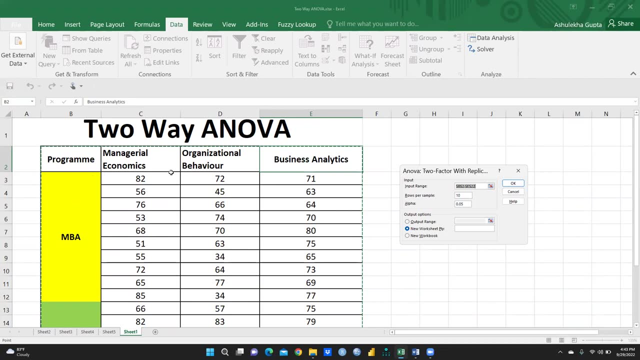 two factor without replication. I am going to use this two factor with replication. I will press okay and this whole data. I am going to select it Rows per sample 10 because in my each sample MBA general program there is the 10 rows data and same with MBA data analytics I have. 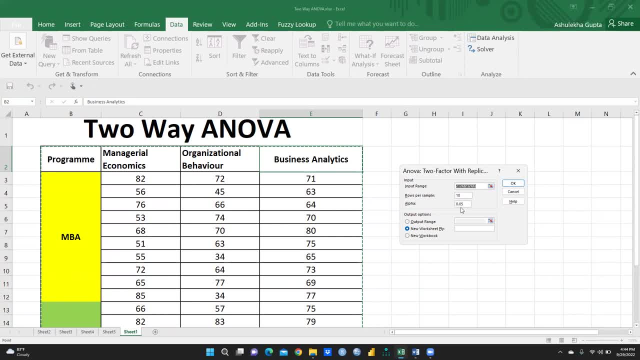 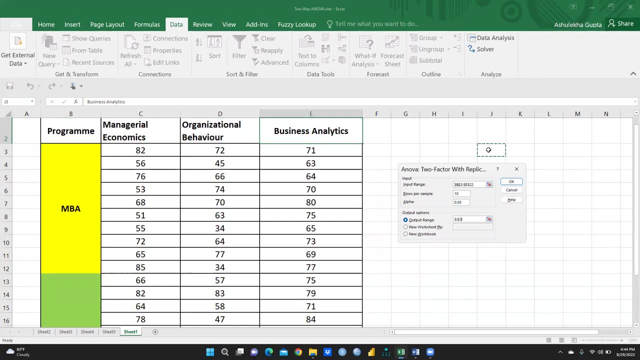 10 rows. Alpha is 0.05.. I want to create this data in my new worksheet. If you would like to have output range here only. so what you have to do, you can just press here and you can click on any row and you have to press ok. So what you have to see is the output range. you can see the output range. 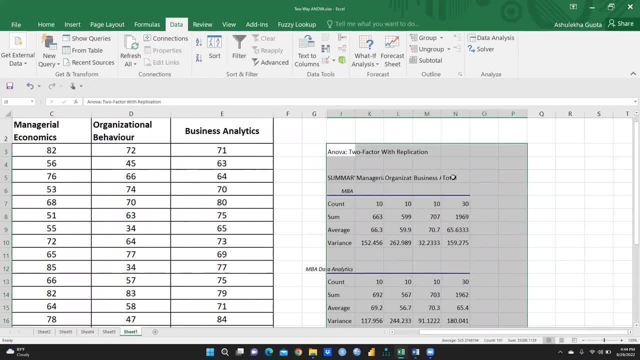 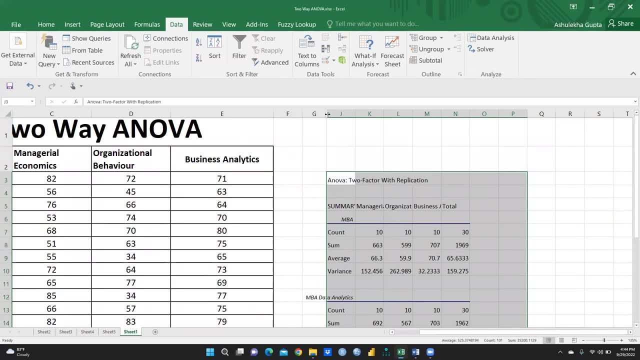 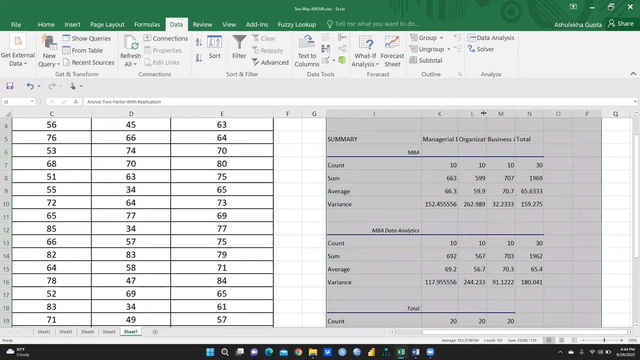 this is the data. now you can see this is data. that is it really? just a moment? yeah, this is my analysis. You can see here ANOVA: two factor with replication. that is the summary, Summary means with all columns and all samples. You can see here these: 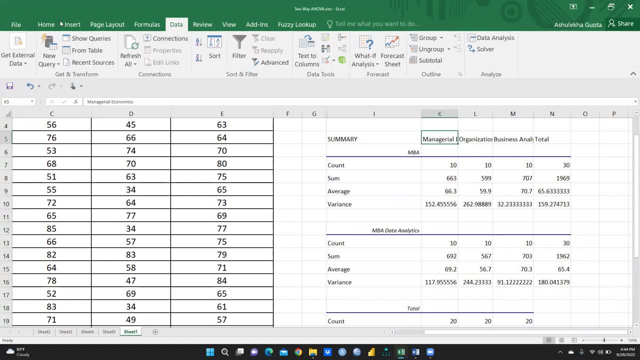 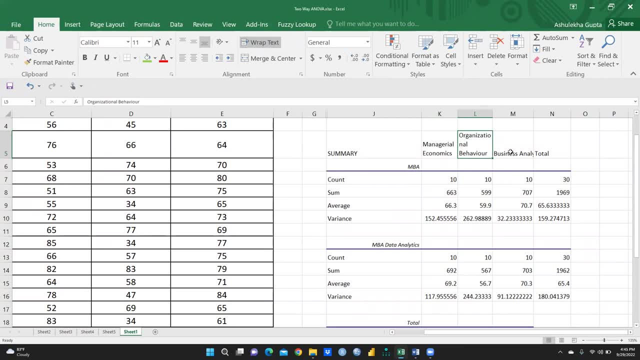 are three columns: First column reflecting first column reflecting managerial economics. Second column reflecting our organizational behavior, and third one is business analytics. Count is 1010 in each subject and total is 30.. Sum is this: the sum of ME marks is 663.. Organizational behavior marks 599.. Business analytics: 707. and. 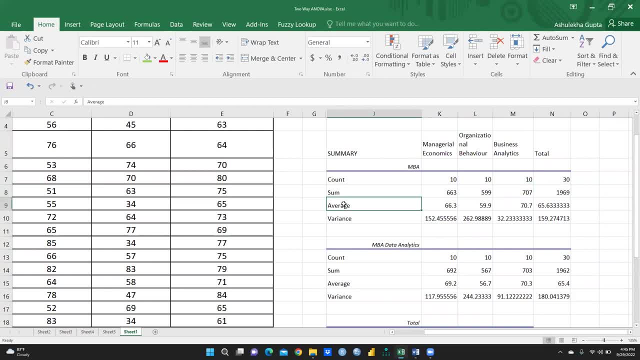 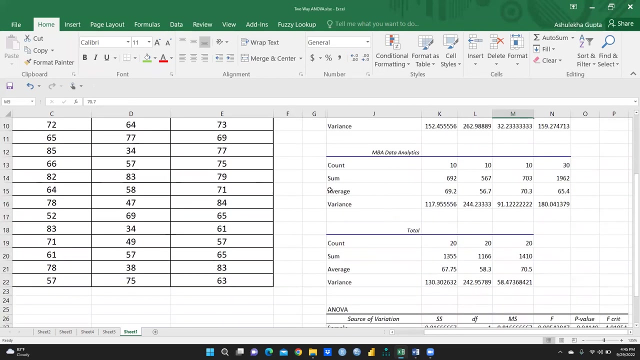 total marks is 1969.. Average- we can compare easily this- managerial economics average marks are 66.3.. Organizational behavior marks 59.9 and business analytics marks 70.7, and this is the variance you can see here And now we come to the. here is this is the summary. MBA data analytics. summary is that: 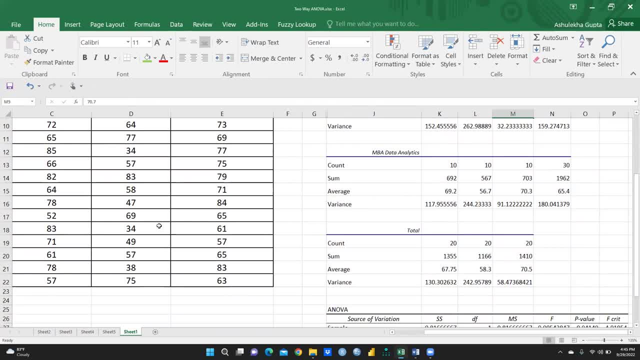 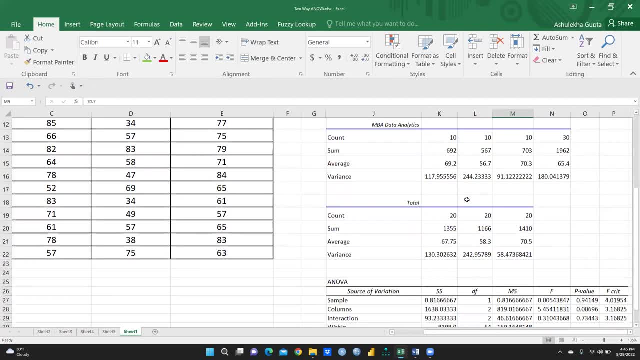 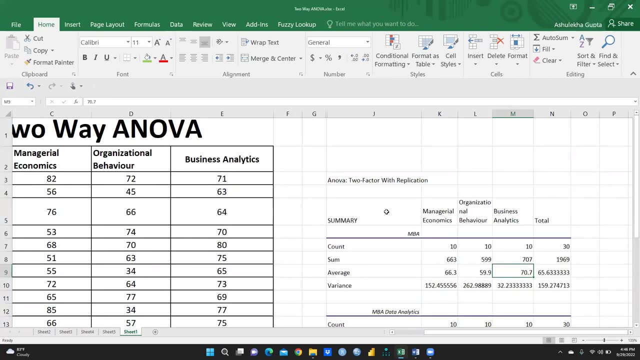 is: that is the entire summary, but this is the only for the next program, that is, MBA data analytics. Count is count, sum, average and variance and total is: This is the total, is this number, and after that we can go for. what do you mean by ANOVA? What is? 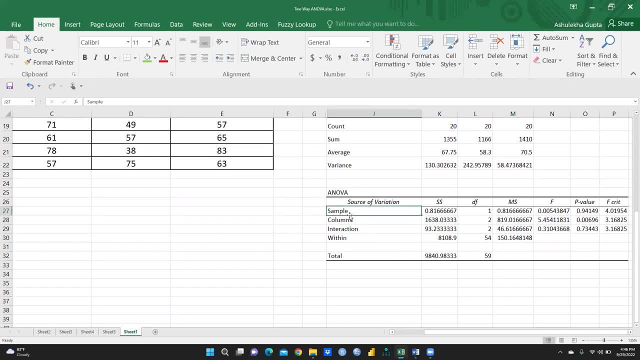 happening here. this is the sample. Sample means we have two samples. Sample A is MBA general and sample B means we have MBA data analytics. That is the right. This is the degree of freedom. mean square F value, P value and F critical. 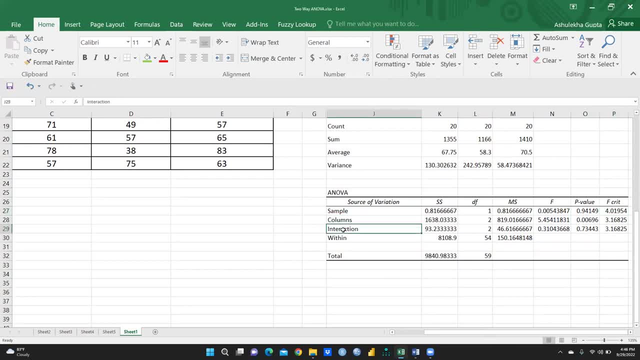 So, and this is the column data, that is the interaction among all the columns with all these programs What we have to do. you can see here we would compare both these things here: F value and F critical value. Here is F critical value. it is greater than F statistics. 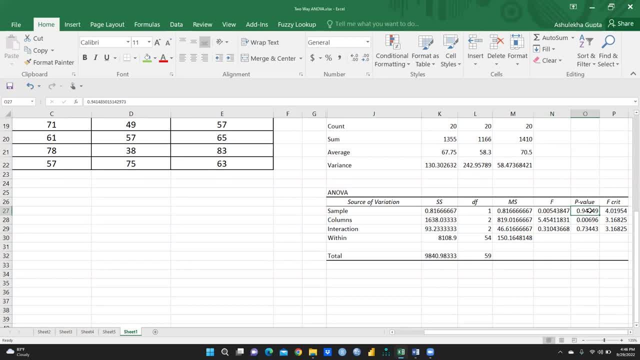 Then the P and P value is higher than 0.05.. That means we are failed to reject null hypothesis. and null hypothesis said there is no difference. there is no difference between both these samples. So that means there is no difference. There is no difference in between MBA and F. 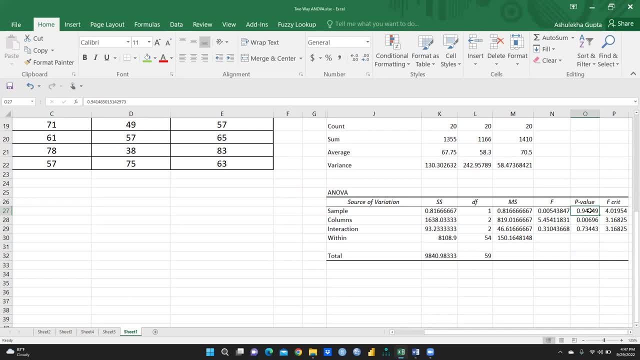 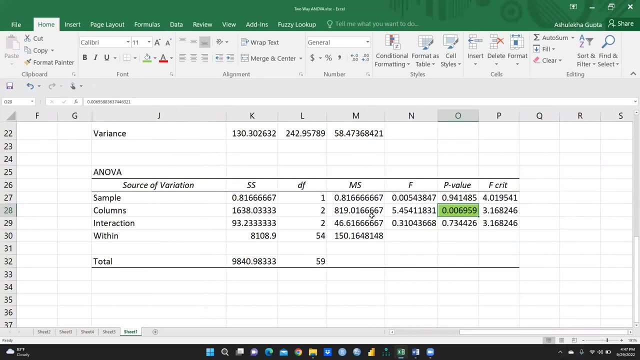 And MBA data analytics as per this hypothetical data, but columns, Columns. you can see here: this is the P value and this P value 0.006.. You can see here, in this value, 0.006959, F critical and this is the F statistics.